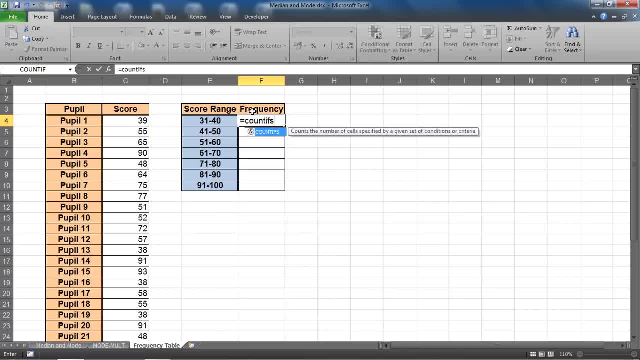 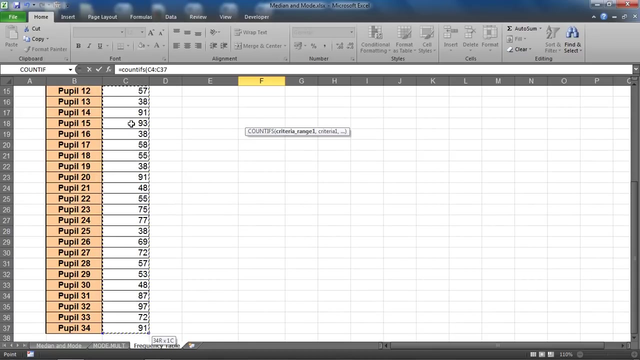 ifs countifs counts the number of cells in a range that meet a given set of conditions, Open in bracket criteria range 1,. what is your first criteria range? That is our only criteria range and it is C4 down to C37.. C4 to C37.. So I can see that. 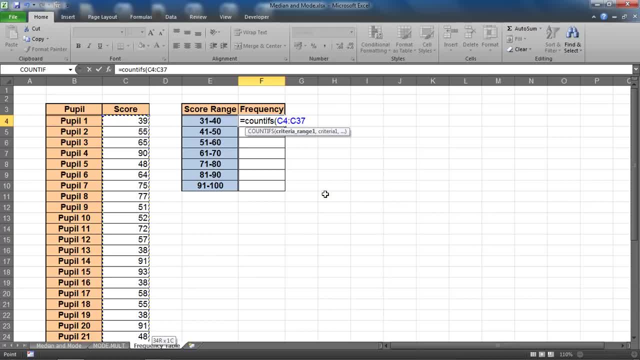 written in the formula bar above as well as there, And I'm going to press F4 to fix that range, Because when I copy this formula to the other cells within this table, I do not want that reference to move. stay in row 4 and row 37.. 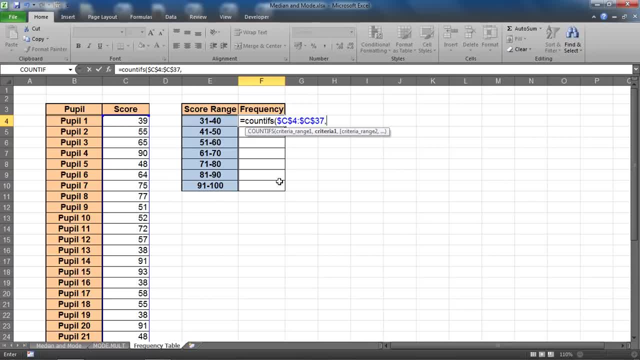 Comma. criteria 1,. what is your first criteria Now in speech marks, all these double inverted commas. we always use them when we use a logical expression within countif or countifs function. I'm going to ask if it's greater than or equal to the number 31.. Because that is the lowest. 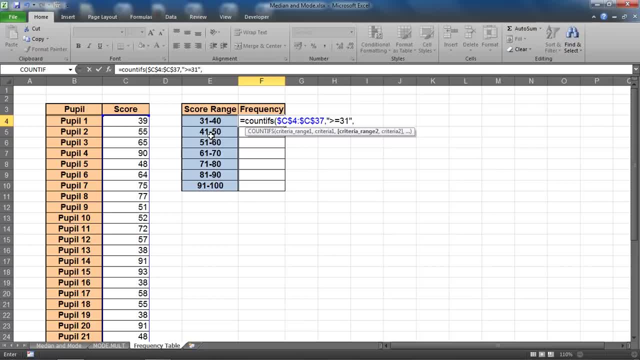 value within that interval, that class. Comma criteria: range 1,. what is your first criteria? Comma criteria 1,. what is your first criteria? Comma criteria 1,. what is your first criteria? Comma criteria 2,. we'll be the same, C4 to C37, which I'll use dollar signs to fix. 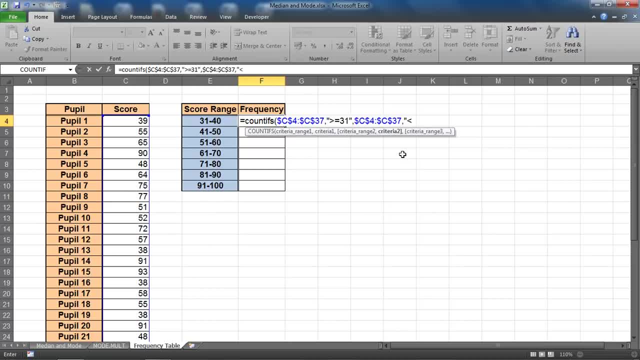 or make absolute, And this time I'm asking if it is less than or equal to 40.. So is it less than or equal to 40 scores? Closing bracket on the end and enter: apparently there are five scores within the range of 31 to 40. now, with that done, 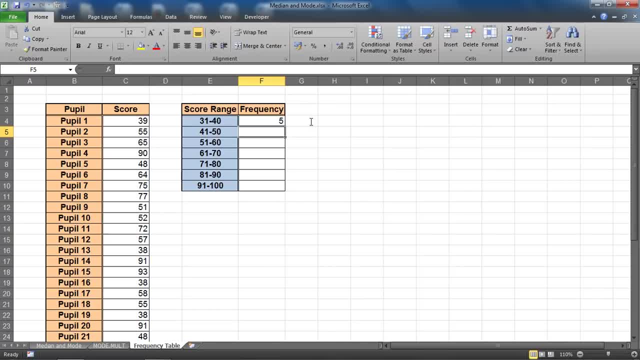 and our reference is fixed. we should be able to copy that formula to the other cells so that references remain looking in the right place but change the range that it's looking within. so that will take a few seconds to get going. but once that is in, jobs are good and we have ourselves a frequency table, all the